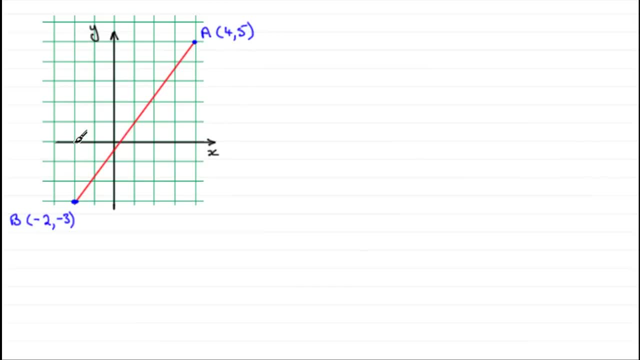 and similarly B is at minus two, minus three. two that way, three down. So how do I find out this distance AB? Well, to do it, what we do is we use Pythagoras' theorem. We think of a right angle triangle drawn something like this, the right angle being at this corner here. 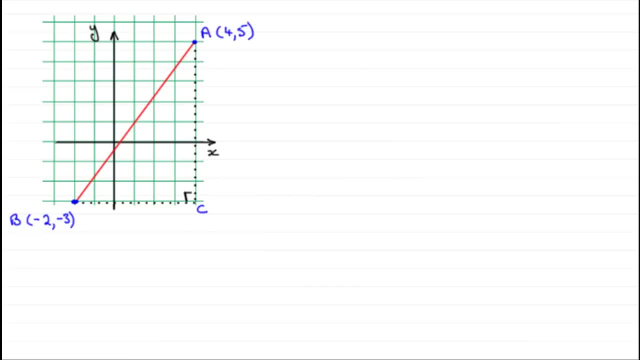 Let's label this C. So what did Pythagoras say? Well, according to his theorem, this side, the hypotenuse, the side opposite, the right angle, that side, the hypotenuse squared is equal to the sum of the squares of the other two sides. 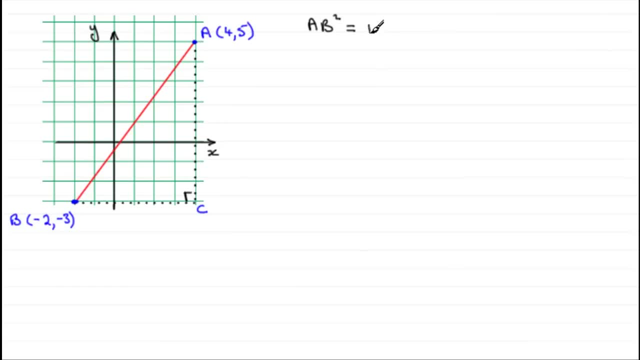 So, in other words, we've got BC squared plus AC squared. Now how do I get the lengths BC and AC? Well, it's very easy. when I've got a diagram like this drawn, You could just simply count squares, You'll see, you've got one, two, three, four, five, six. 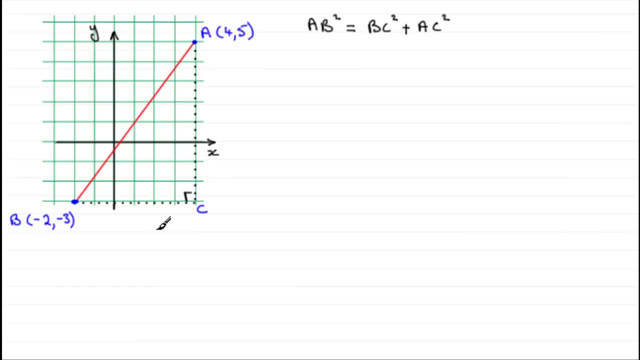 Six units this way, And for this one AC it's just going to be one, two, three, four, five and three, down here eight. But suppose we hadn't got this diagram drawn? How can we work it out then? 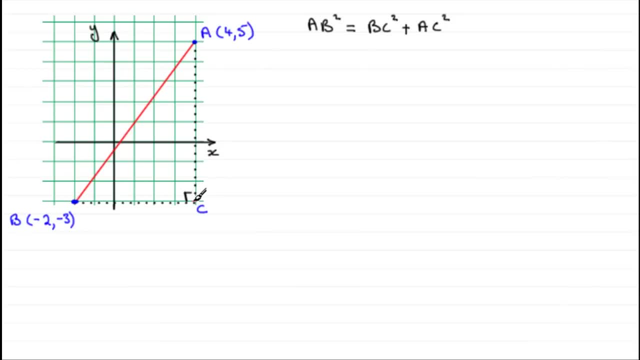 Well, what we can do is that this distance, BC, is given by the difference between the X coordinates, In this case four minus the minus two here, Four minus minus two, Four minus minus two is six, And it works for AC Because we do the difference between the Y coordinates, the five and the minus three. 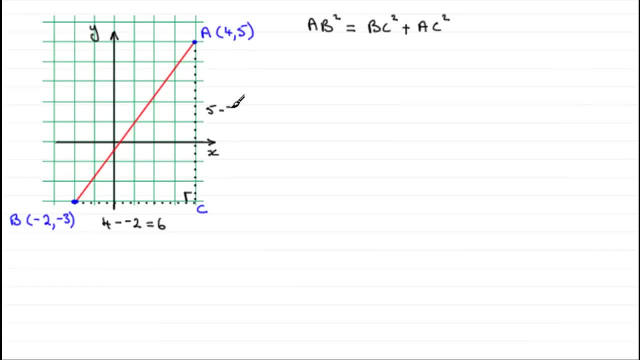 Because five minus minus three gives us five plus three, which is eight. So when it comes to working this out, the length BC is going to be then four minus minus two. That's the difference in the X coordinates By Pythagoras' theorem. we have to square it though. 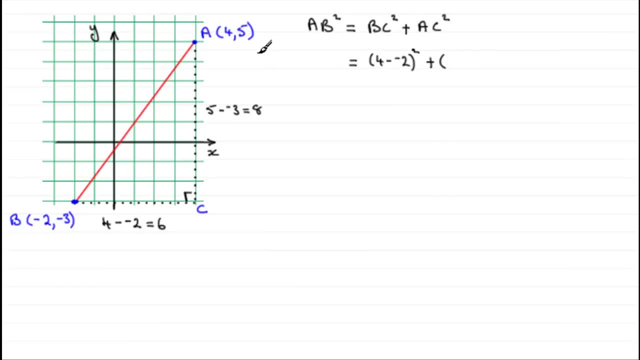 And for AC we do the difference between the Y coordinates, five minus minus three, And we square that. So what we have here is that we have six squared, which is thirty-six, And eight squared, which is sixty-four. If we add these two together, we get a hundred. 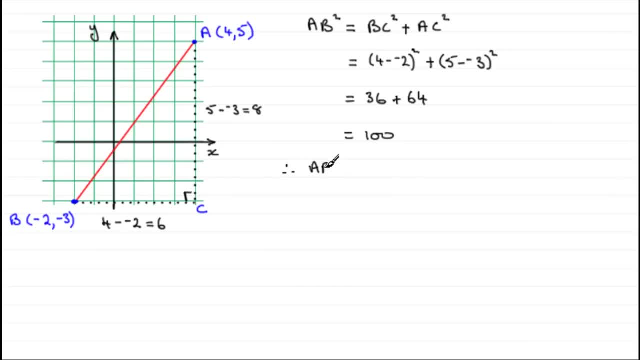 And then to get AB, what we need to do is do the square root of a hundred, which is clearly ten, And we're dealing with a length, And it's not measured in centimetres, in this case, or metres, It's just units. 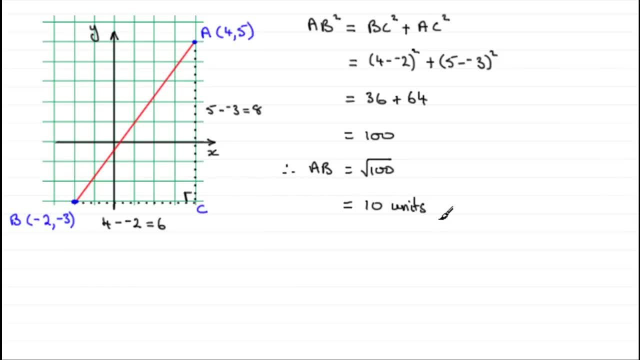 So I like to put units on the end if I'm finding a length. You don't have to put that. Quite often you'll find that's not quoted in answers in textbooks, But I just like to put that in Now. I'm often asked: does it matter which way round you subtract your X coordinates and your Y coordinates? 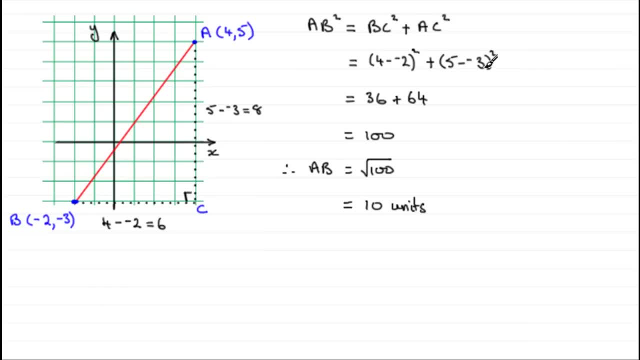 Will you get the same answer. Well, let's try. Instead of doing four minus minus two, suppose we did minus two minus four. What would that give us? It gives us minus six. OK, you can't have a length, that's minus six. 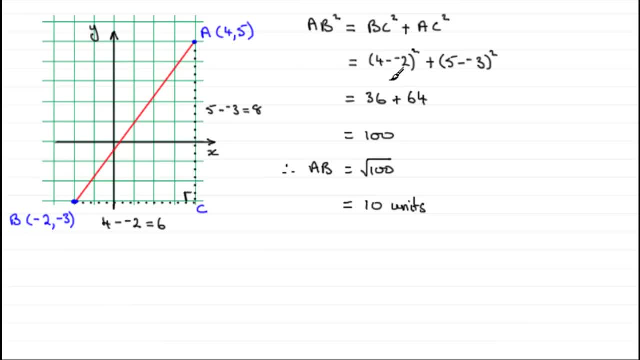 But by Pythagoras' Theorem you're going to end up squaring it anyway. And minus six squared still gives you thirty-six. And the same applies to the difference in the Y coordinates. If, instead of doing five minus minus three, you did minus three minus five, you'd get minus eight. 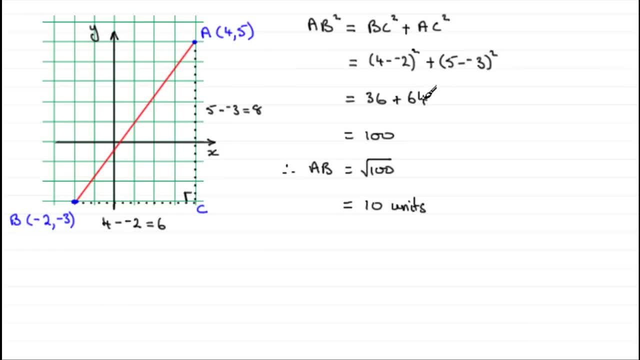 But when it comes to squaring minus eight, you're going to get sixty-four anyway. So it doesn't matter which way round you subtract your coordinates, As long as you do the difference in the X coordinates squared plus the difference in the Y coordinates squared. 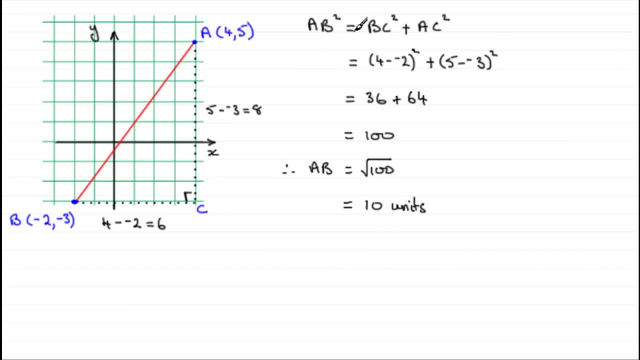 OK. Well, that's given us a numerical example. What about an algebraic, a general result? Well, if we had our axes, Let's just mark them on Our X axis and our Y axis, And we had any line. 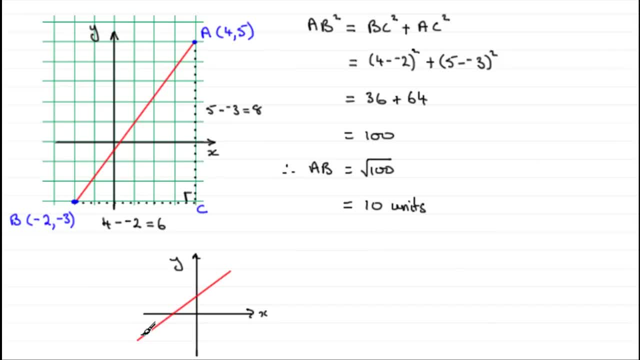 OK, Two points on the line. Let's say this point is A and it's got coordinates X1, Y1.. And another point here, B, And it has coordinates, say, X2, Y2. Then by using Pythagoras' theorem, we don't really need to draw this triangle in. 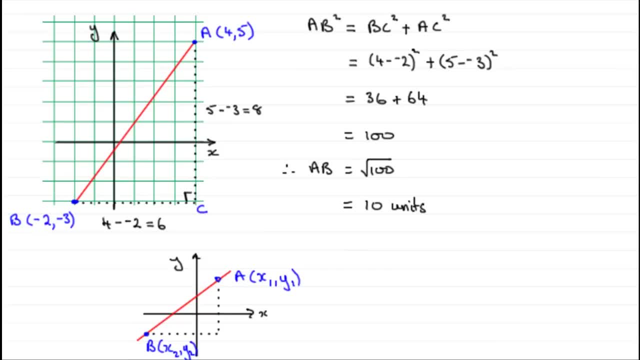 But at least it helps in the thinking process. Then to get AB, AB squared is equal to the sum of the squares of the lengths of the other two signs. So in other words, The difference in the X coordinates X1 minus X2.. 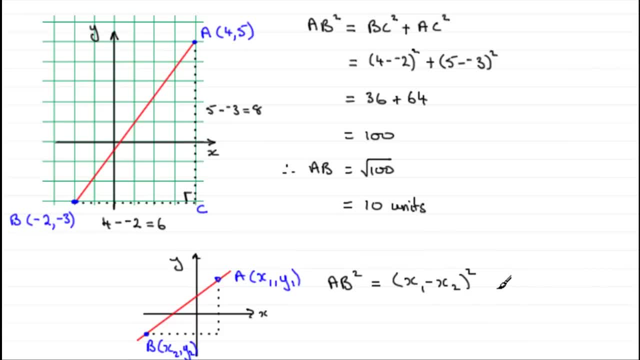 Or X2 minus X1.. Doesn't matter, because we're going to square it Plus the difference in the Y coordinates. And again I'm just going to say Y1 minus Y2 squared, But you could say Y2 minus Y1.. 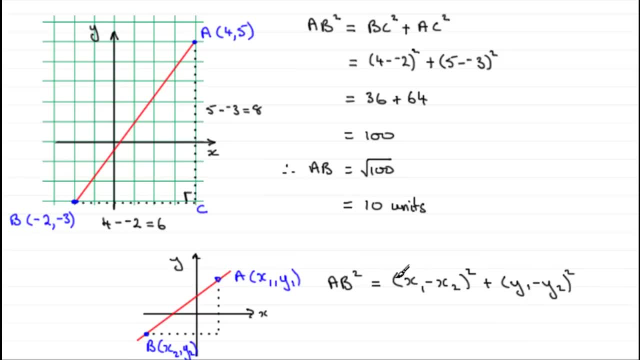 Doesn't make any difference. That's AB squared. When it comes to finding AB, we need to square root both sides, And the square root of this is just going to be AB. And for the square root of this side, well, just mark in the square root sign. 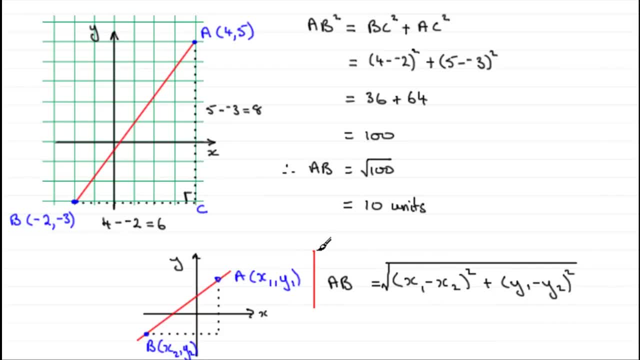 And it's that formula that I would encourage you to learn and understand. Understand that it's coming from Pythagoras' theorem. OK, Well, I'm going to do a numerical example for you now, OK, Or you might like to try it. 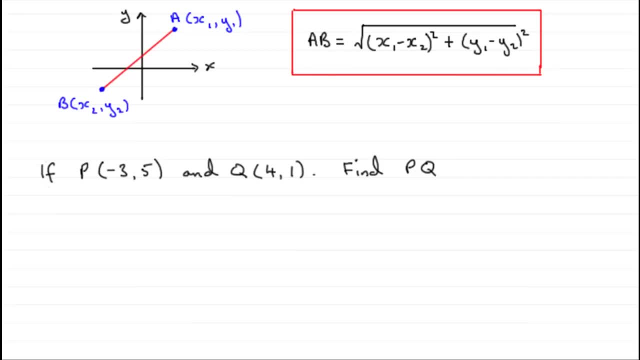 OK. So here we've got our question. If P has coordinates minus 3,, 5. And Q has coordinates 4, 1. We've got to find the distance PQ. So we know that to find PQ, All we need to do is the square root of the difference between the X coordinates squared. 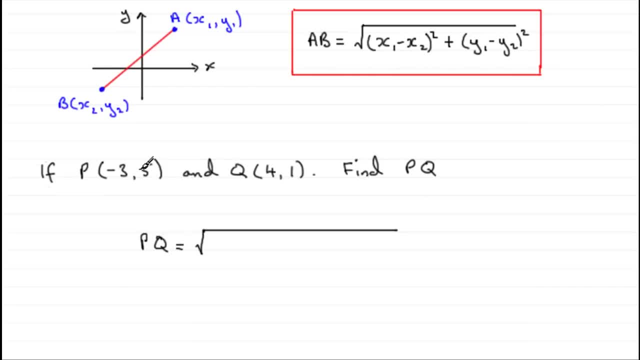 Plus the difference between the Y coordinates squared. So I'm going to take minus 3.. Put it in brackets: Minus 3. And then subtract the 4. And then we square that Plus the difference in the Y coordinates. So we're going to do 5 minus that 1..